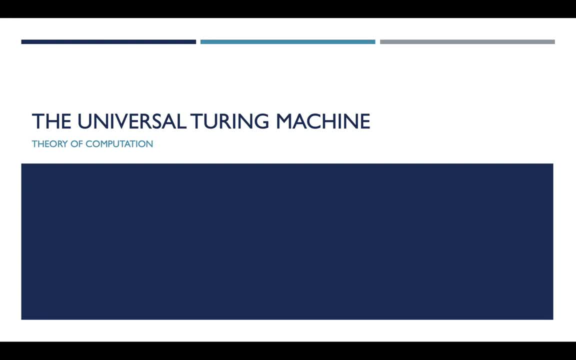 And basically what we're going to do is show that you don't necessarily have to have a Turing machine for every algorithm. You can have one Turing machine that runs or simulates a whole bunch of different Turing machines that actually implement those algorithms. And so we'll get started. 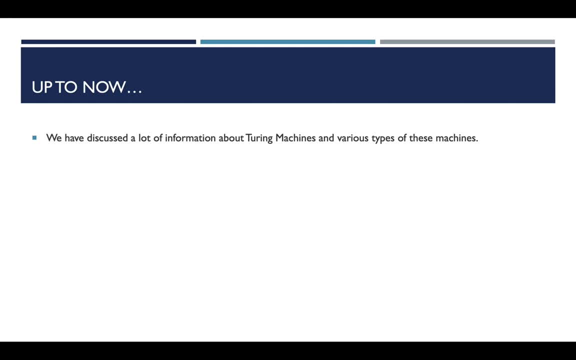 So, up to this point, what we've done is we've talked a lot about the various formats of Turing machines and a whole bunch of different things that they can do, And we've talked about how Turing machines are in some ways equivalent to algorithms, using the definition that we derived. 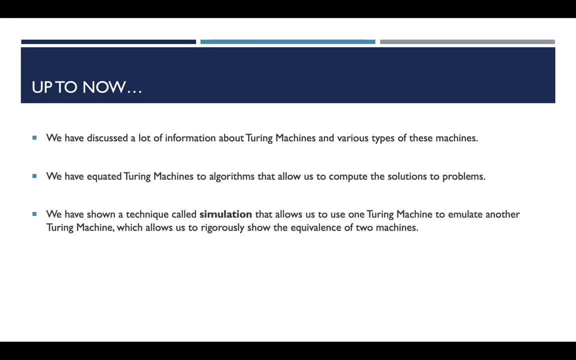 From Turing's thesis. So what we used to show that two Turing machines can be equivalent, so all the different variations of a standard Turing machine can be equivalent. We showed that through something called simulation, And this idea is that I can have a Turing machine that then emulates a different Turing machine and that gives us the ability to mathematically rigorously show the equivalence. 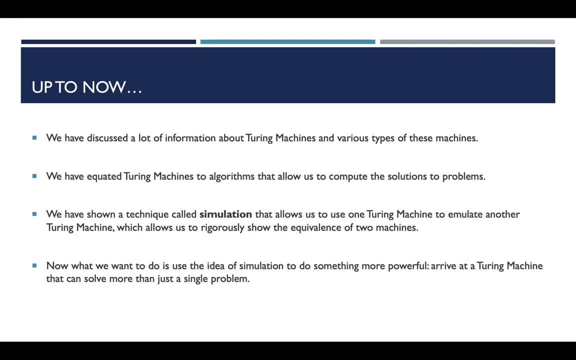 which is the Turing machine. So what we want to do now is take these last two bullet points and sort of merge them together. What we want to do is take a single Turing machine and we want to use that Turing machine to simulate all other Turing machines. 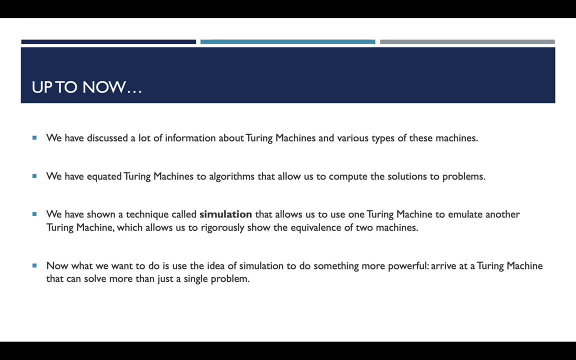 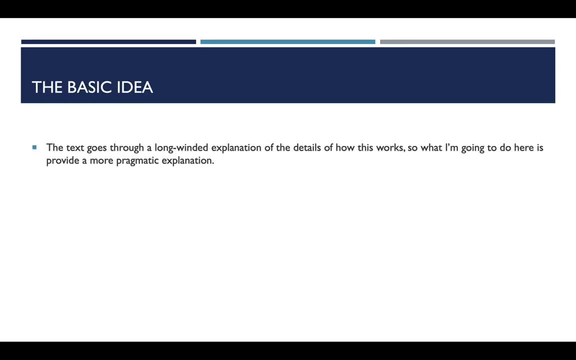 which amount to algorithms that we can run on our simulator or our universal Turing machine. So the basic idea of this is exactly that We're going to build one Turing machine. That Turing machine is going to have a transition function that allows us to go through all of the different possible states in a Turing machine that is provided as input on the tape. 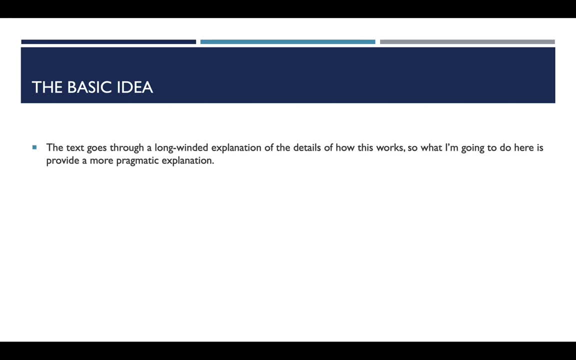 And that's going to be that. And so, while the textbook spends three or four pages trying to convince you that this is a thing that you should care about and this is a thing that can be mathematically rigorously derived, what we're going to do in the video is we're going to try to provide a little bit more information about what we're going to do in the video. 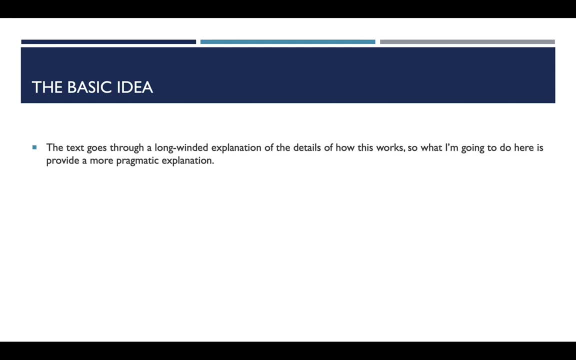 So we're going to try to provide a little bit more information about what we're going to do in the video And we're going to do a little bit more of a pragmatic explanation, so you get both And so hopefully that's helpful. So previously we have shown the equivalence between a Turing machine as an algorithm. 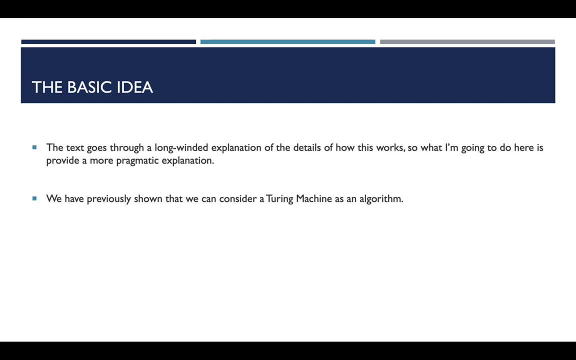 And so we did that, I believe in the part two video of Turing machines. I think that's probably lecture number 22 or something like that, Or 21,, rather probably. And so because we know that Turing machines are algorithms, 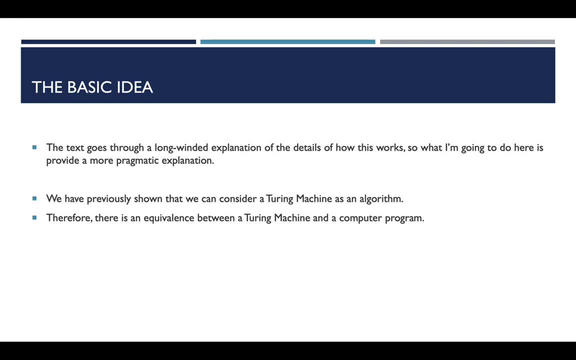 algorithms or Turing machines implement an algorithm, be it for membership in a language or even arithmetic, like we showed in a previous example. we know that there is therefore some sort of equivalence between a computer program, as you can write it in a higher level language like C++ or Java, and a Turing machine as a low level concept. 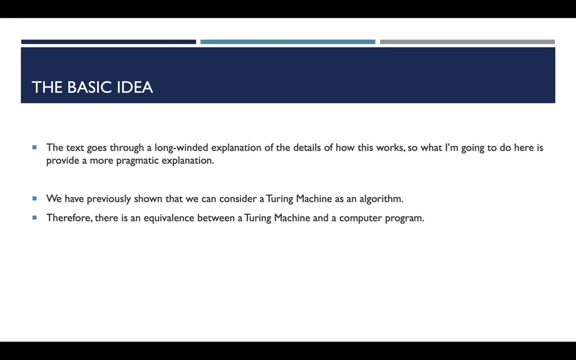 And so anything that you can do with a Turing machine according to Turing's thesis, you can do the digital computer and vice versa. So what we're doing here is we're expanding that equivalent between a Turing machine and an algorithm to a Turing machine and a computer program like the ones that you have created. 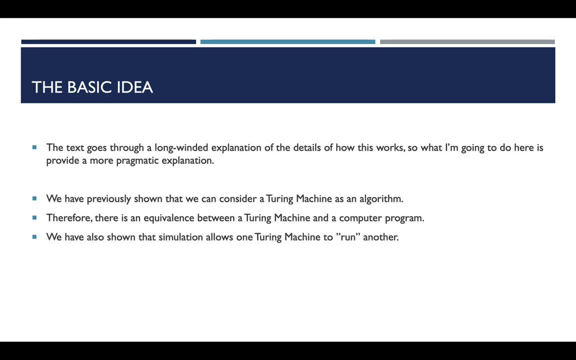 for programming assignments through your other courses. So we have also previously shown that if you have two Turing machines and those Turing machines have equivalent power, you can simulate one on the other and vice versa. So what we can do is we can create a result there as a global current powered assignment. 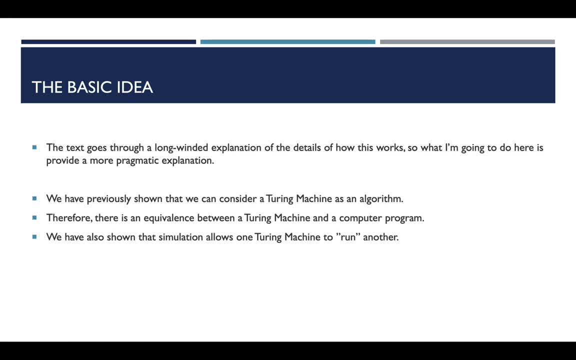 going over that one format in the software magically and then pulling it directly into a staircase, a Turing machine that is capable of simulating another Turing machine, and the Turing machine that's being simulated is effectively just an algorithm. So we can think of the simulator. 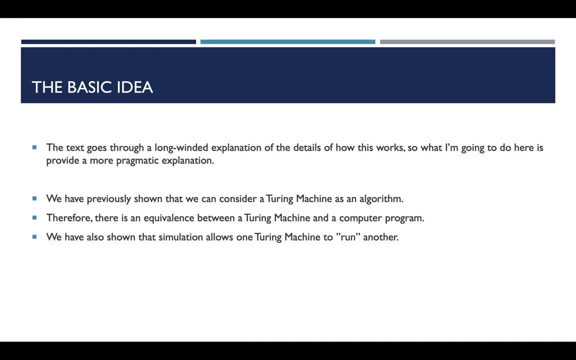 Turing machine as a computer, as a digital computer that is actually running some sort of compiled executable code. So a universal Turing machine is a machine that allows the simulation of any arbitrary Turing machine that solves some problem, And so this fits the bill of a machine that's much closer to a digital computer or a general purpose machine. 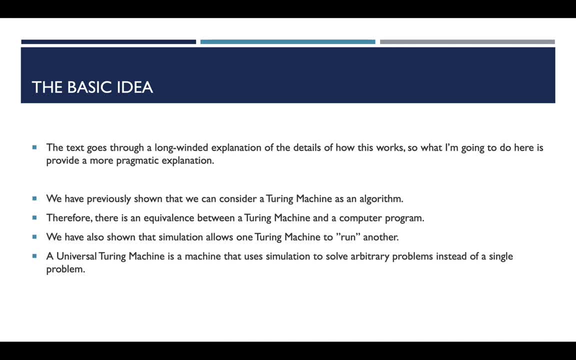 like the one that you're watching this video on, And so what we want to do in this lecture is not necessarily build a simulator for a specific, a single Turing machine or a single algorithm. What we want to show is that there exists a universal Turing machine that can. actually run a Turing machine, And so what we want to show is that there exists a universal Turing machine that can actually run a Turing machine. And so what we want to show is that there exists a universal Turing machine that can actually simulate any Turing machine. 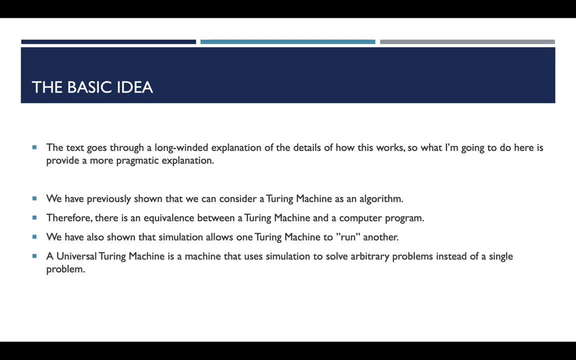 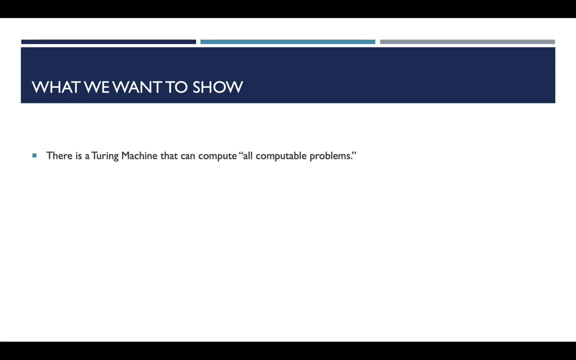 And so, therefore, that universal Turing machine is effectively a general purpose computer. So, in a kind of mathematical way or sense, what do we want to show here? What we want to show is that there exists a Turing machine that can compute, quote, all computable problems. 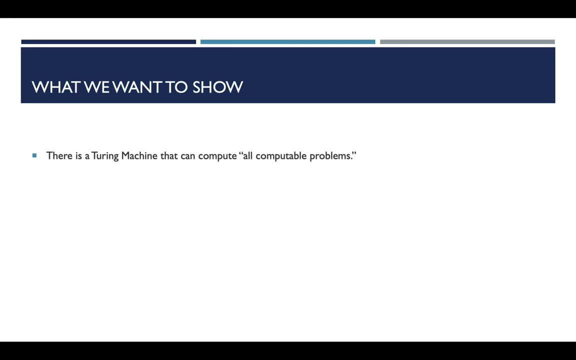 And so these quotes go back to Turing's thesis, And basically what we want to show is that basically, the outcome of that is that what we want to do is show that there is a Turing machine that can simulate all other possible Turing machines, including itself. So you, 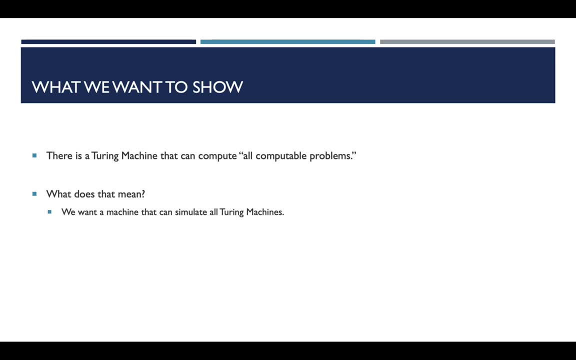 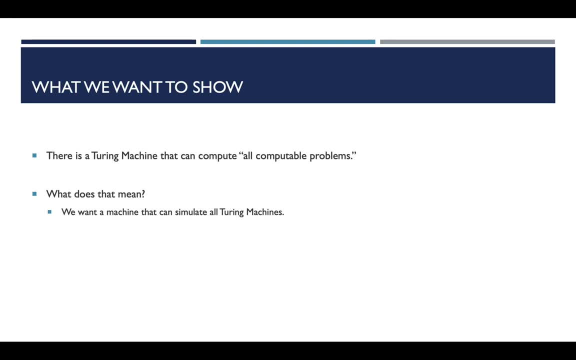 You can have a virtual machine that runs inside of a virtual machine, that runs inside of a virtual machine that runs on your physical desktop or your physical laptop, And so this concept of a universal Turing machine extends to basically anything that we have discussed previously as a thing that a Turing machine can compute. But you can also, kind of colloquially, 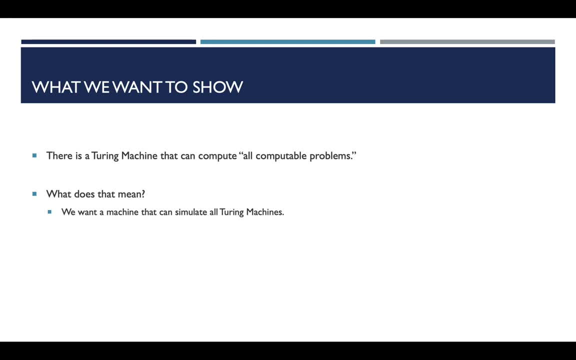 think about it as anything that the machine that you're working at right now can compute, So it feels plausible that you could do this right. We've seen several, several examples of how you can simulate one Turing machine on another at this point, But the biggest. 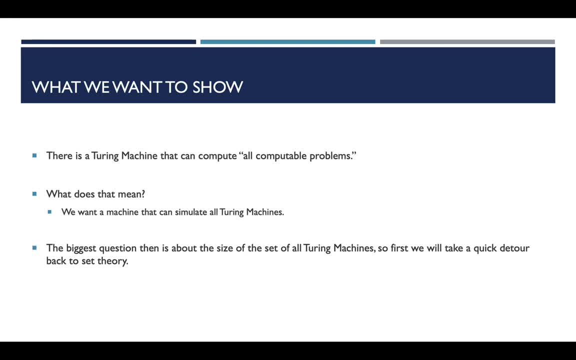 question that kind of throws a wrench in this whole works is the size of the set of Turing machines. So the problem is what happens if there are uncountably infinite Turing machines? There is no real way to show that we can go through them in any sort of ordered fashion. and then 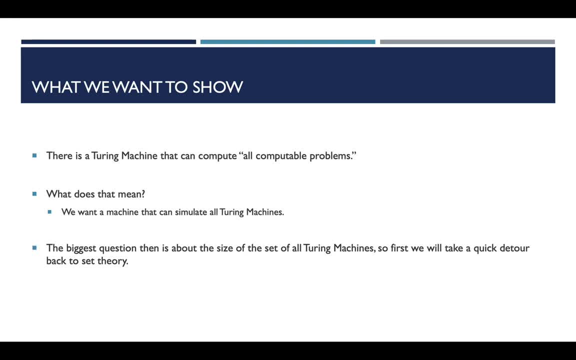 run each of those Turing machines. So prior to actually talking about the computational theory part, we need to go back and take a detour to set theory. So we mentioned this in the very first lecture in the course and we've used this a couple 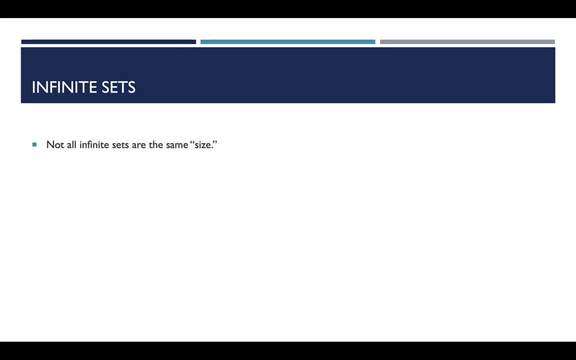 of times since. One of those times was when we were talking about the pigeonhole principle for pumping lemma. But it's true that not all infinite sets are the same quote size. There are various cardinalities of infinite sets, And a countably infinite set is a set. 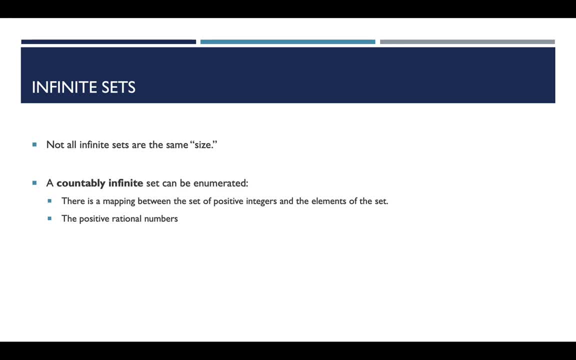 that can be enumerated. So what enumeration effectively means is that you can take each of the elements in that set and you can map it to a positive integer So you can effectively number all of the elements of that set. So even if your set goes to infinity, you can. 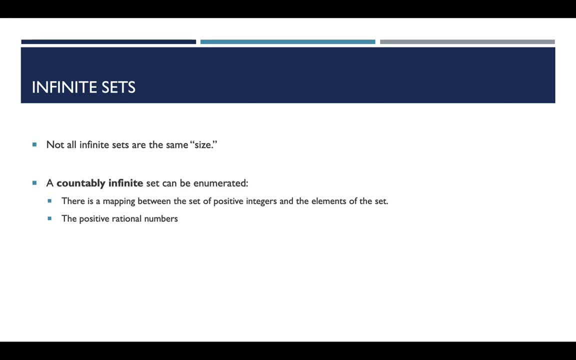 always draw a line between an element in that set and an element of the positive numbers, And it has to be a one-to-one mapping. An example of this is the positive rational numbers, And so, if you remember from Discrete 2, you can use a Tantor set or a similar and equivalent. 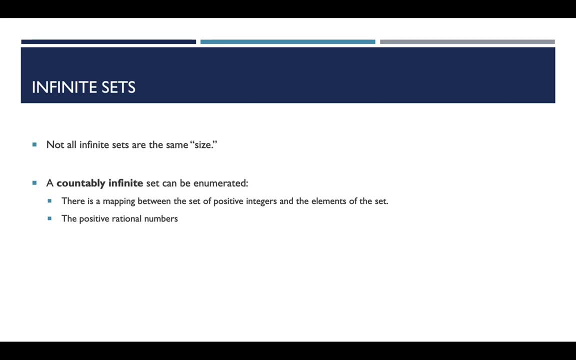 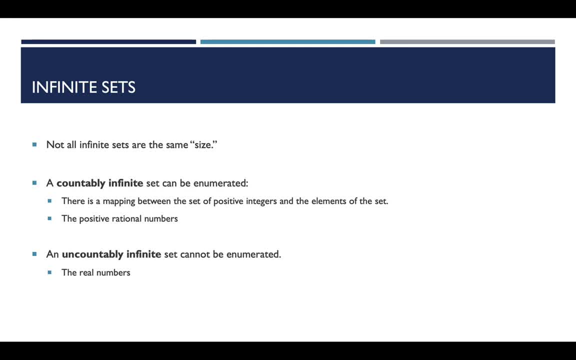 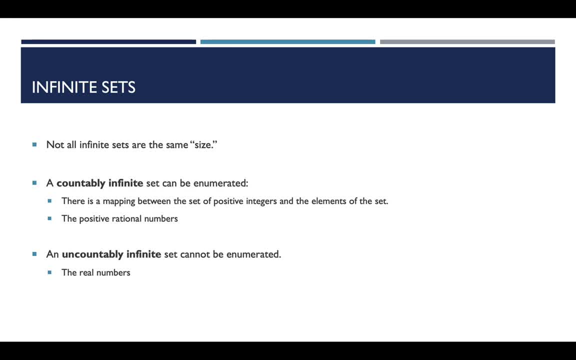 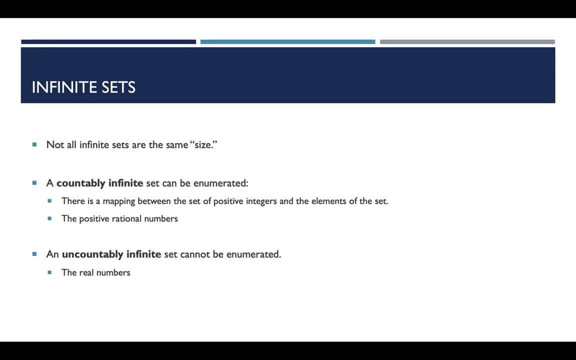 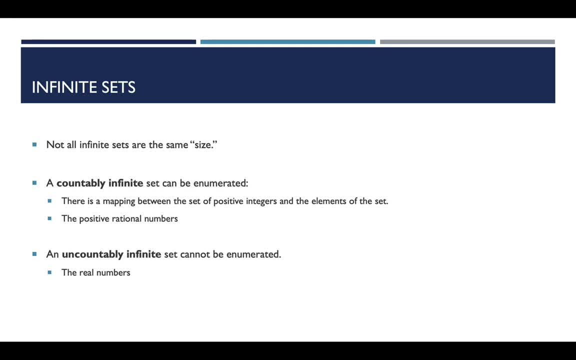 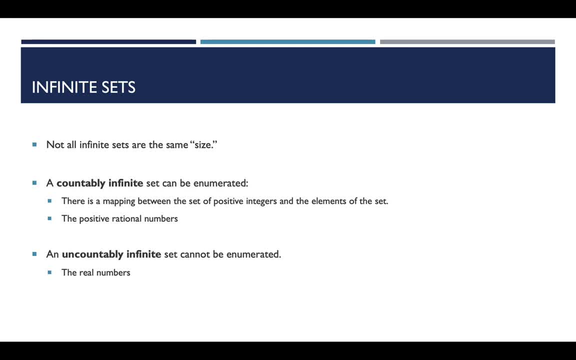 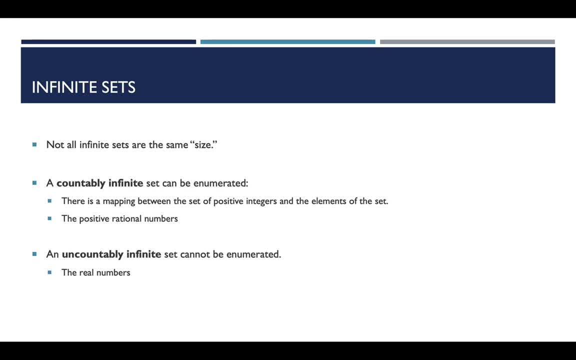 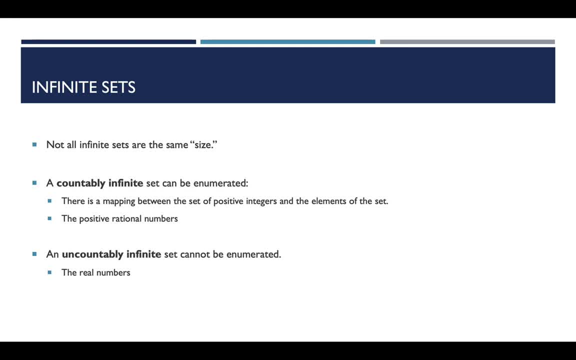 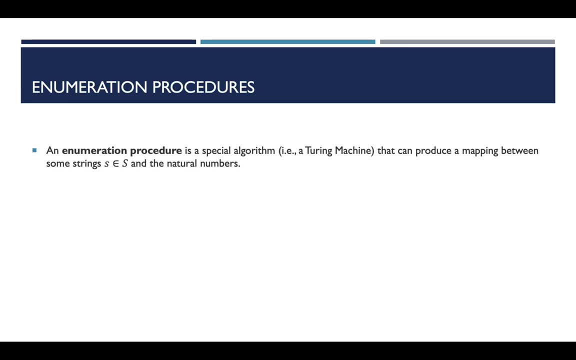 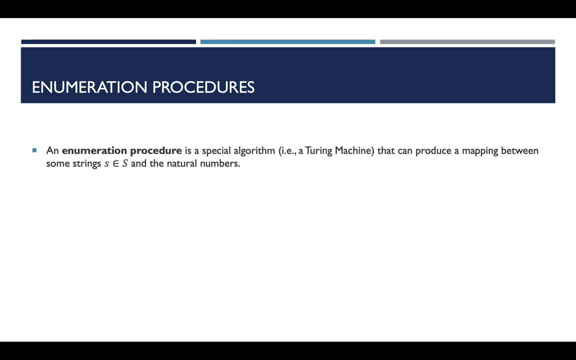 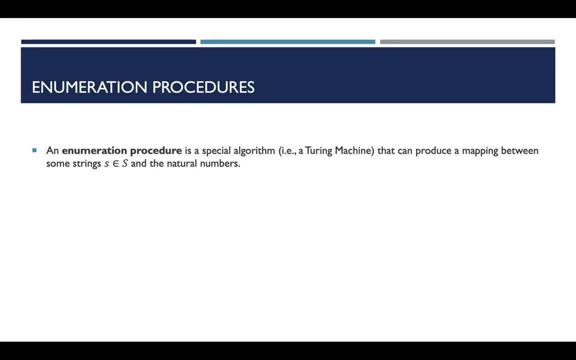 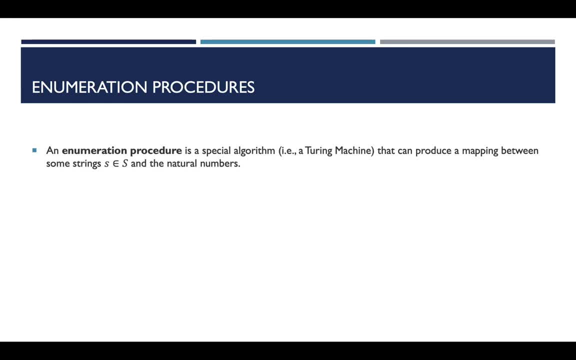 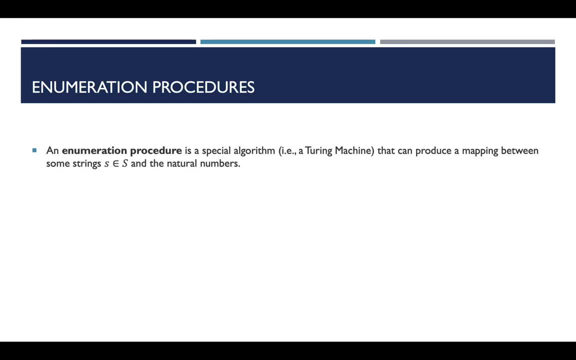 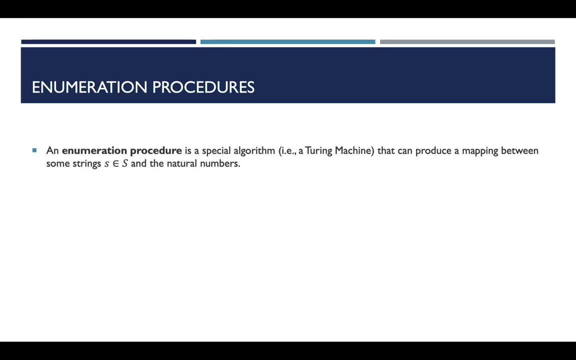 Turing machines are really onwards. This is ağlju ćitñaj čizečける trepanщxx jouž. conferences of the element in the set corresponds to the natural number that the element is map to", And so we can recall that during a simulation, effectively all we're doing is we were taking 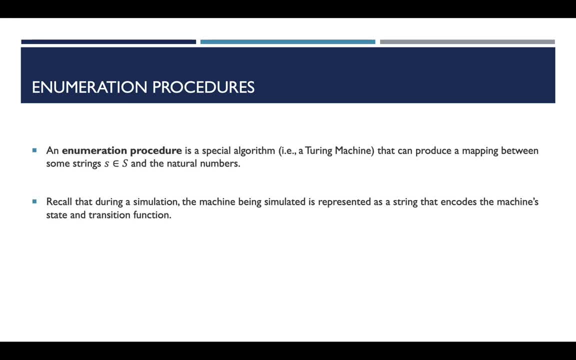 some string representation of a Turing machine. so we are taking the internal states, taking the transition function itself, And we're taking the input characters in the alphabet and we're putting that onto the tape for a simulator and then we can simulate the machine on the tape with that Turing machine that is reading it. 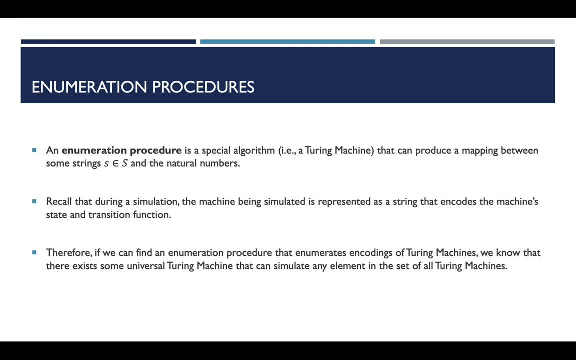 So basically, what we need to show here is if we can find an enumeration procedure that enumerates all the possible encodings of Turing machines. we know that there is some universal Turing machine that can then simulate that element, and that element corresponds to one of the possible Turing machines, and we're kind of done. 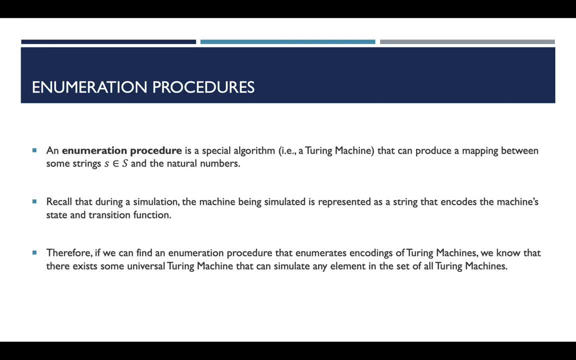 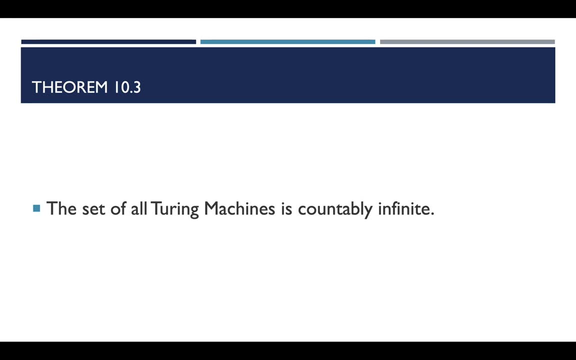 We've showed that there exists a Turing machine that can go through and simulate all, All possible Turing machines, because we can enumerate the list of all possible Turing machines. So the theorem that all of this stuff hinges on is labeled 10.3 in the text and it effectively just says that the set of all possible Turing machines is countably infinite. 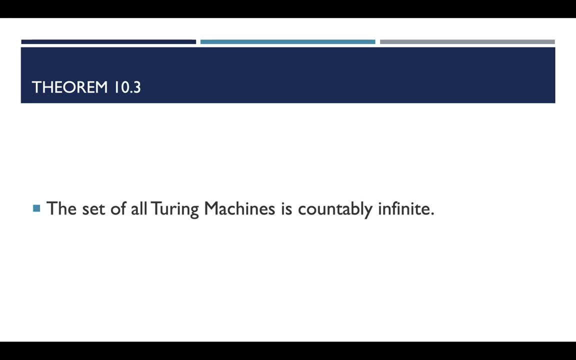 So what this is saying is that if I have a set of all the possible Turing machines in the world, or in the universe, or in existence, I can count them. I can count them by ascribing each one of them a positive integer. 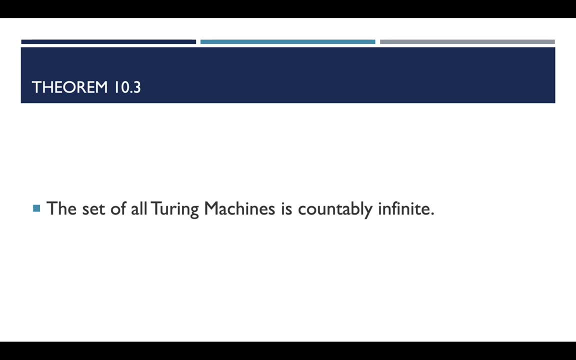 What that means is that we can now go through and enumerate that list with a Turing machine and then use that same Turing machine- or a different Turing machine- to actually simulate each of those algorithms And from a mathematical perspective. what that means is we have created a machine that can understand which of the 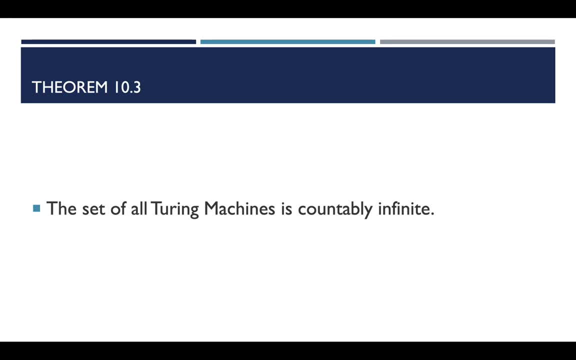 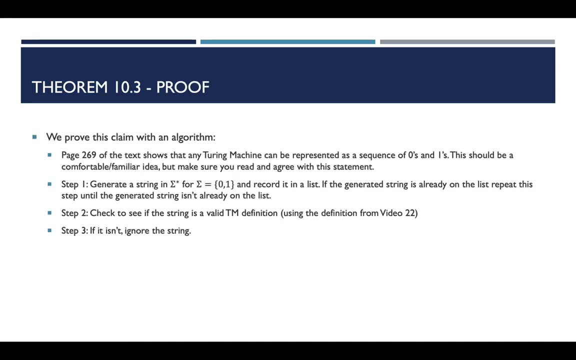 strings or string representations, is a viable Turing machine and then for each of those viable Turing machines can actually simulate it. So we can actually prove this thing with a proof or with an algorithm or with a step-by-step sort of procedure. 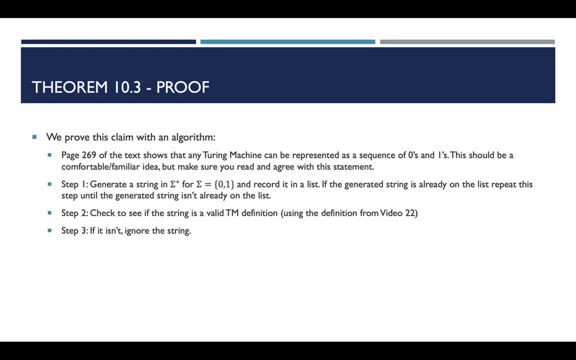 So if you look at page number 269 of the textbook, it shows in just a couple of- maybe a paragraph and a half, a couple of sentences that all the possible Turing machines can be represented as a sequence of zeros and ones. 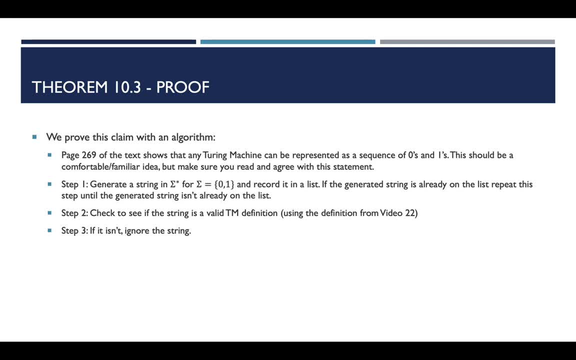 And just based solely on digital representation. this should be a fairly comfortable or familiar idea, But what I would do is just make sure that you read that maybe five or six sentences and convince yourself that that's a real thing. Effectively, what they're saying is: you can derive any. 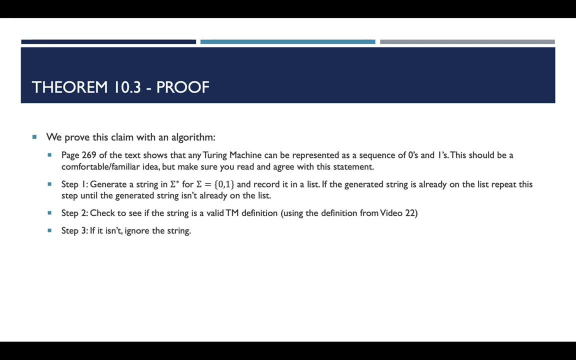 any structure that you want, Any string that you want, be it an alphabet symbol, alphabet of Cyrillic symbols or capital Roman symbols or whatever. You can represent all of those things with a binary string And within that binary string, you can always use a unique binary representation of a spacer. 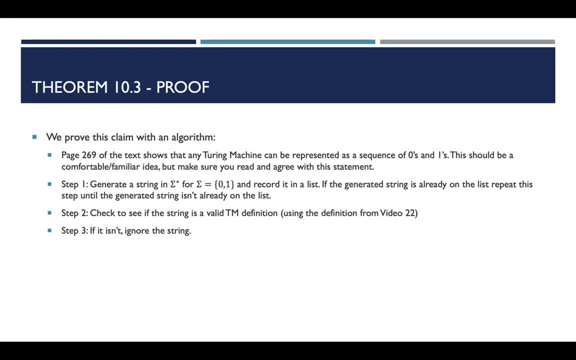 And so each of those spacers can tell you which part of a Turing machine you are currently reading. So, for example, The transition function will have a special starting delimiter, a special ending delimiter. The internal states, or the possible states, will also have special delimiters. 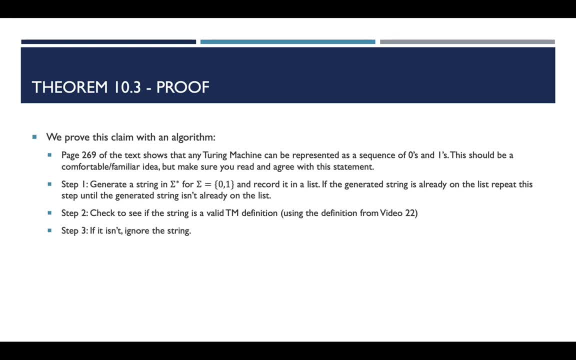 Each of those things will be represented by a unique combination of zeros and ones, And again, that should be fairly familiar because that's effectively how everything is represented on a digital machine anyway. So the process that we're going to use to actually prove this theorem: 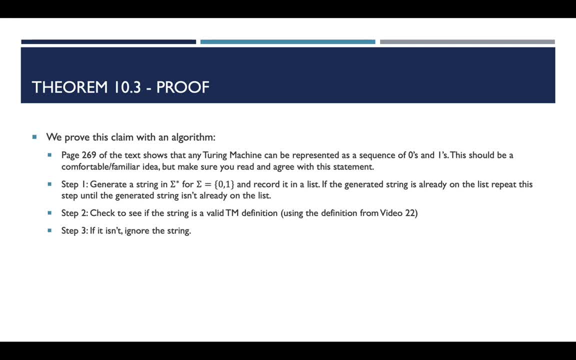 We're going to take an alphabet that only consists of zeros and ones, And note: this would also work for something that isn't zeros and ones, if you can show that those alphabet symbols can be used to represent any Turing machine. So there are many, many, many alternatives to this. 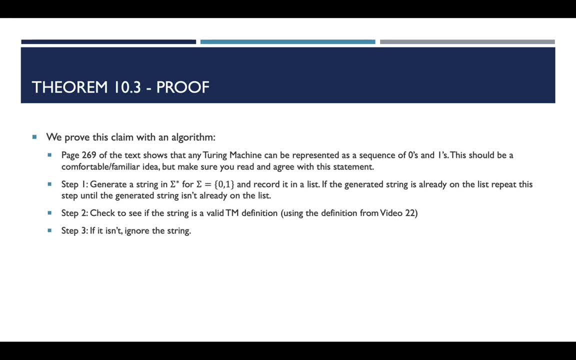 But what we're going to do is start generating all of the possible strings in the clean closure of an alphabet consisting only of zeros and ones. So what we're going to do is we're going to generate that string and we're going to store it in a list. 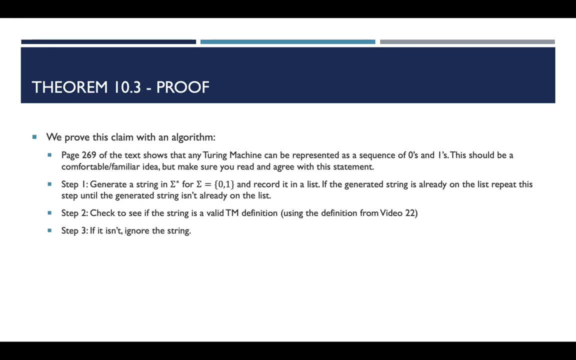 If we attempt to store it in a list and that list already contains that string, we just go to the next one. We generate another string and another string, and another string and another string, until we find a string that hasn't already been added to the list. 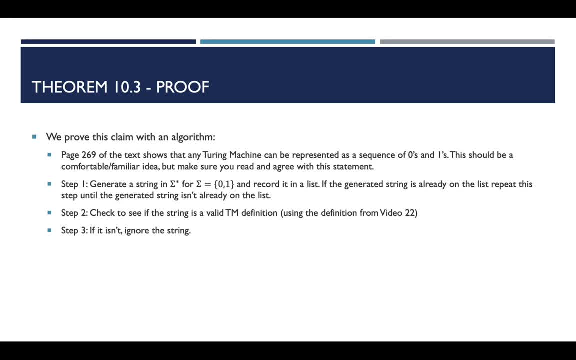 So in step two, what we're going to do is we're going to check to see if the string, if the string itself, is a valid definition of a Turing machine, And we can do that using the definition and using the example from video number 22.. 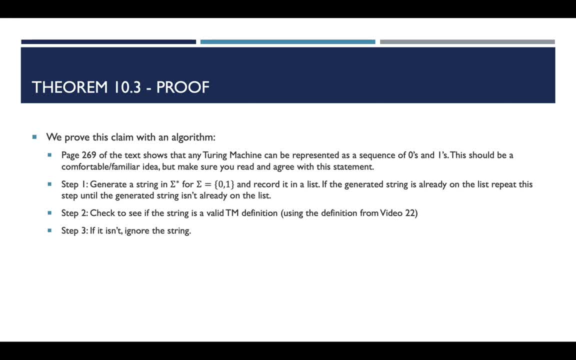 Effectively, what we're going to do is we're going to say: does this thing have a valid transition function? Does this thing have a set of internal states? Does this thing violate any of the mathematical definition terms of a Turing machine? But you can also think of this as syntax checking from context-free languages. 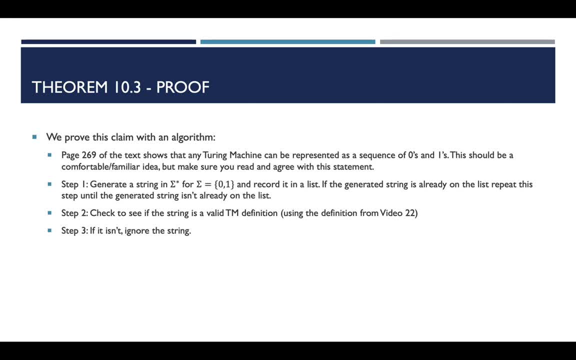 Right, And we can look at if the algorithm itself is coded in the appropriate language. We can tell if a C++ program is missing a closing brace somewhere, We can tell if a Java program is not well-formed, etc. etc. So if we determine that the Turing machine definition is valid, we can then simulate that Turing machine. 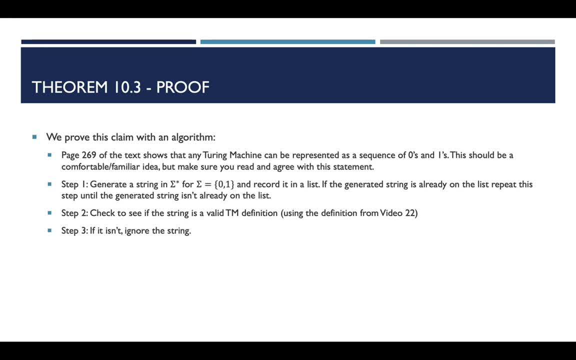 and we're done with that. We're done with that particular algorithm. We've shown that effectively anything can be, or any Turing machine can be, simulated by another Turing machine as long as their power is equivalent. And so, after simulating that Turing machine, we can go on and on and on. back to step one. 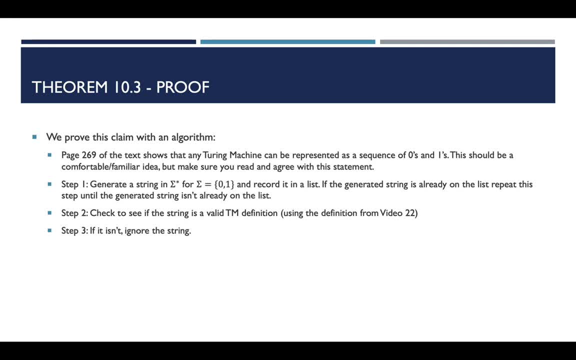 If the Turing machine is not a valid Turing machine, then we're going to ignore the string and proceed back to step one and continue on about our lives. And so this algorithm never terminates right, Because we could potentially always find the next algorithm or we could find a new Turing machine. 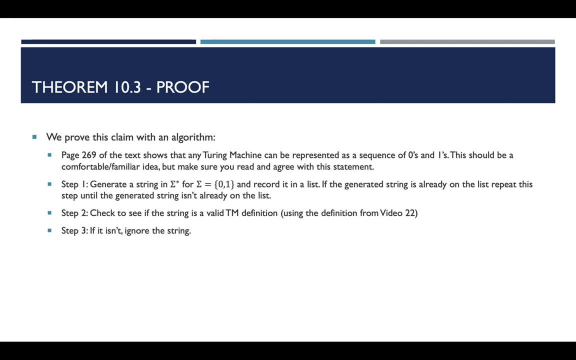 because the set of Turing machines is always, or has been shown to be, countably infinite. But any time we arrive at a valid Turing machine definition, we have shown that you can actually simulate that Turing machine, And so we can kind of orderly go through these Turing machine definitions. 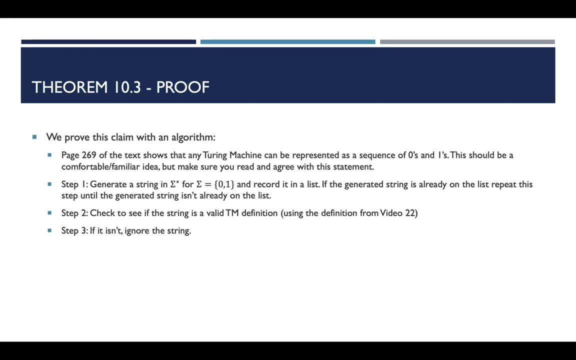 And in the list that we're creating in step one, the index of that element in the list is the enumerable mapping, And so the very first algorithm that we simulate is the zeroth position or the first position, The second one is the first or the second, so on and so forth. 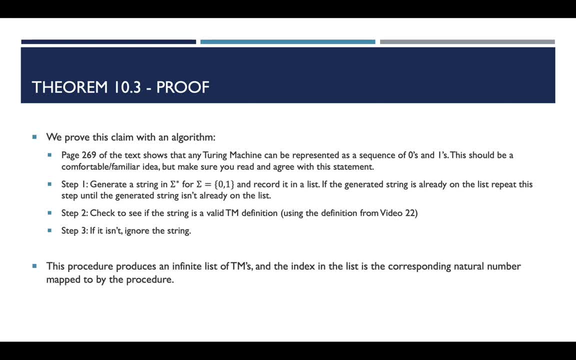 Depending on if you're using zero or one base counting, And so, like I said, even though this procedure is producing and simulating an infinite list of Turing machines, we always have an index in that list that maps us back to the natural numbers. 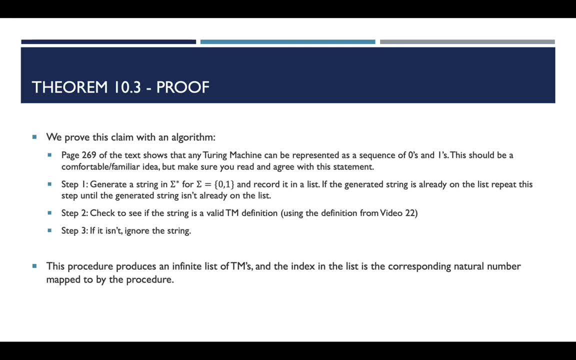 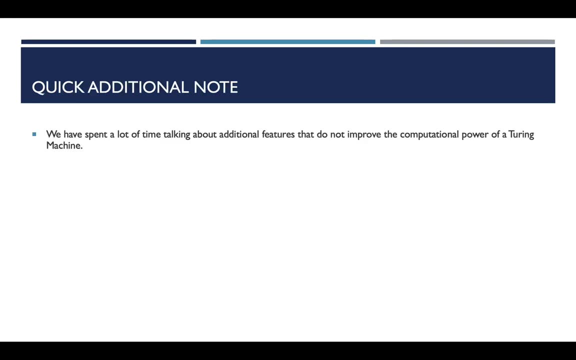 And that is consistent with the fact that the Turing machine list is a countably infinite set which we were given by, which is really actually the theorem we're trying to prove here. So a quick additional note about this is: we have spent a very long time talking about all the different features that you could add to a Turing machine. 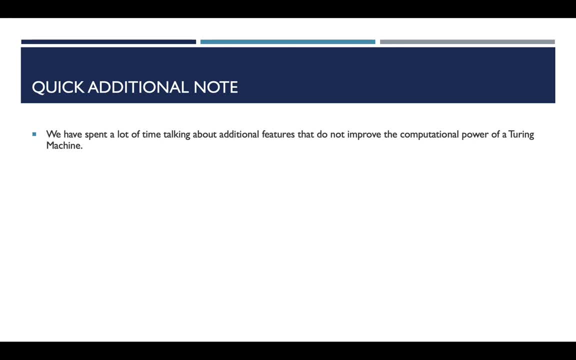 We talked about multiple types of storage, We talked about multiple ways that you could improve the read-write head and all of that kind of stuff, And the high point of that is that all of those modifications were such that you didn't actually improve the computing power of the machine. 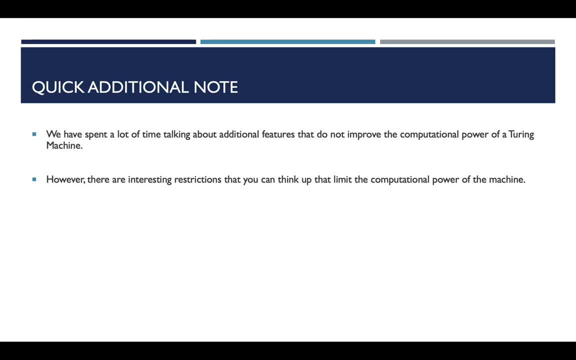 The interesting thing, though, is there is the flip side of that coin. There are actually things that you can do to a Turing machine to restrict it and limit the computational power of the machine, And there are some interesting properties that you can come up with. 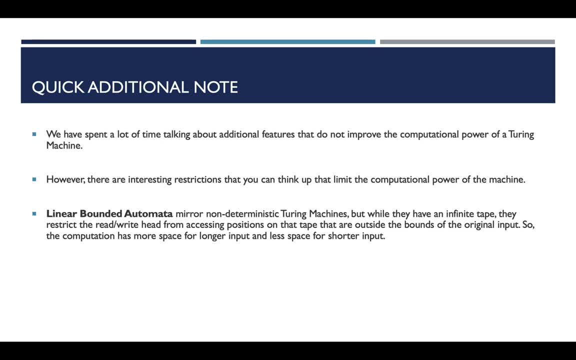 And the biggest one, or the one that is really highlighted. the one that is really highlighted by the text is called a linear bounded automata, And basically what this means is you have a non-deterministic Turing machine And that Turing machine begins with some input on the input tape. 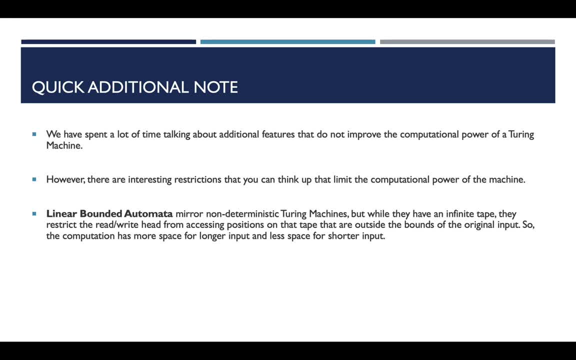 Let's say that it is 10 symbols on the input tape. A linear bounded automata works the exact same way that a non-deterministic Turing machine does. It allows you to go through multiple or a transition relation to multiple different states or multiple different configurations. 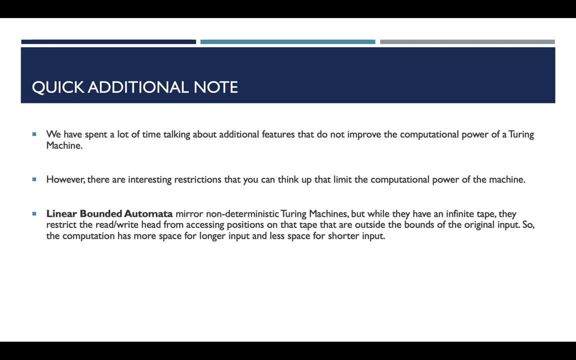 But it does not allow the read-write head to exceed the bounds of the original input string. So if you have a really, really long input string, you have much more space than if you begin with a very, very short input string And there are some kind of language restrictions. that this pleases. 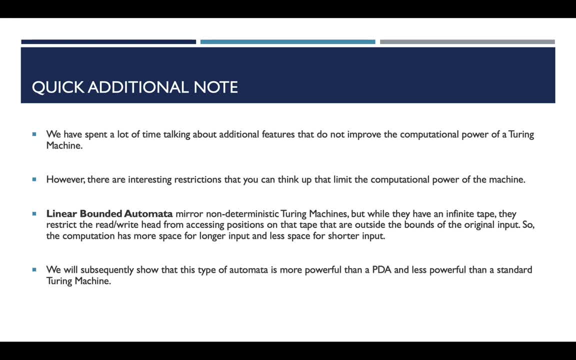 that we're going to talk about in the next couple of videos. So the important thing to note right now is that we have talked about language families previously, And so we talked about regular languages. We talked about context-free languages. We're shortly going to be talking about context-sensitive languages. 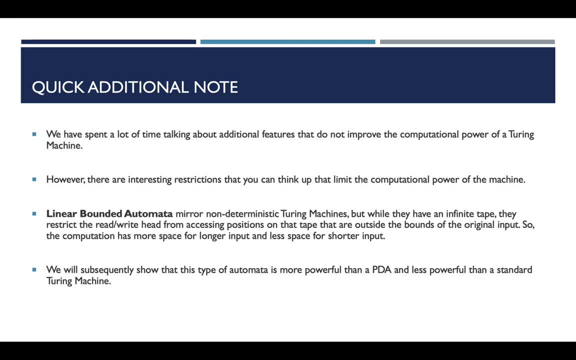 And so what linear bounded automata do is? they represent a series of languages or a language family that exists between PDAs and Turing machines. So they are slightly larger than the set of context-free languages, but it is smaller than the languages that are accepted by a Turing machine.